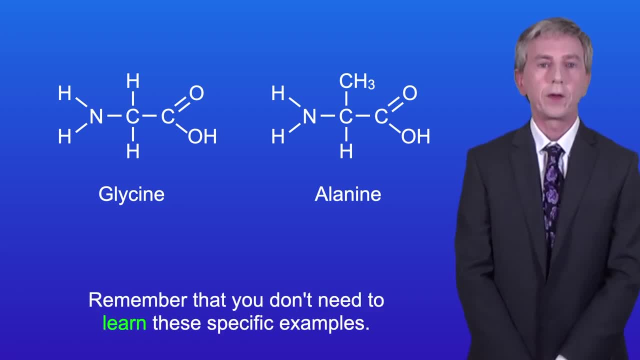 different amino acids here and remember that you don't need to learn these specific examples. In the case of glycine, the R group is a hydrogen atom, and in the case of alanine, the R group is a carbon atom bonded to three hydrogen atoms. Now in the exam, you could be asked to name the elements. 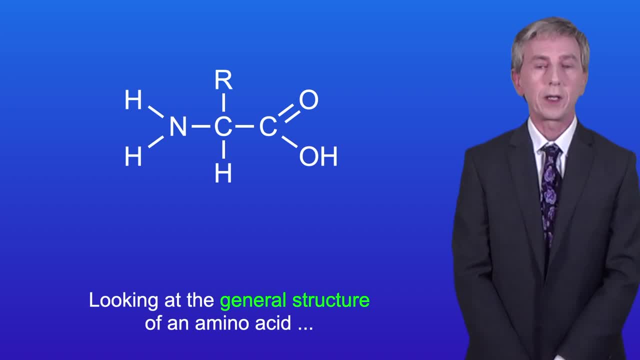 present in proteins. Looking at the general structure in amino acid, we can see that they contain the elements carbon, hydrogen, nitrogen and oxygen. Some amino acids also contain the elements sulfur Coming up. we're going to look at how amino acid molecules can bond together. 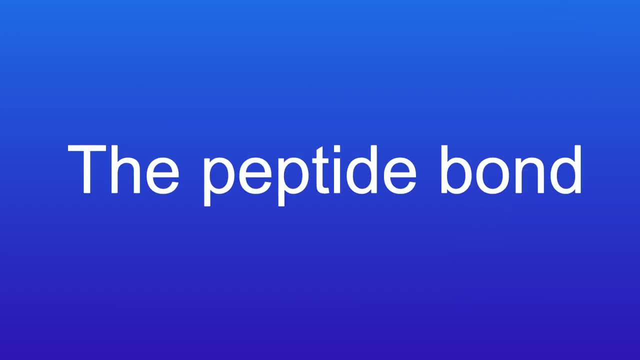 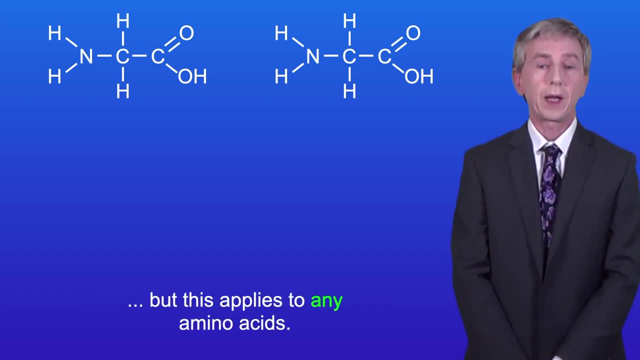 by forming a peptide bond. Okay, I'm showing you here two amino acids side by side. In this case, these amino acids are both glycine, but this applies to any amino acids. Now, these two amino acids can react together and form a chemical bond, and I'm showing you that here. 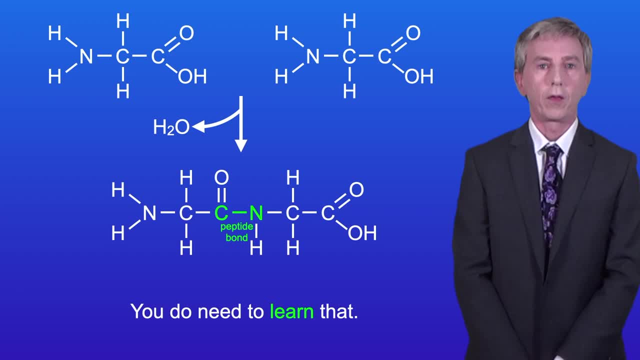 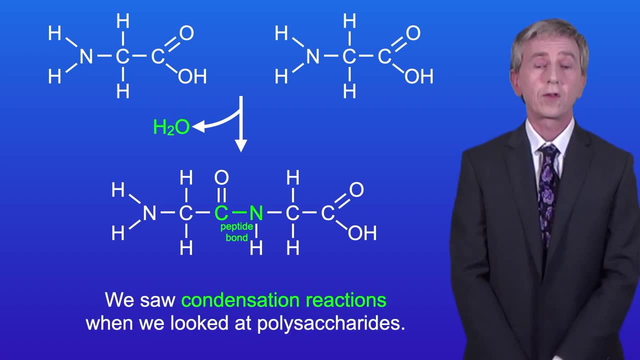 The bond formed is called a peptide bond, and you do need to learn that. As you can see, we've also formed a molecule of water, so this is an example of a condensation reaction, and we saw condensation reactions when we looked at polysaccharides. The molecule that we formed is called a dipeptide, as 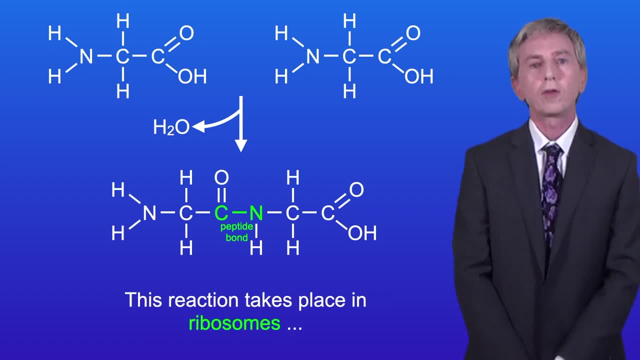 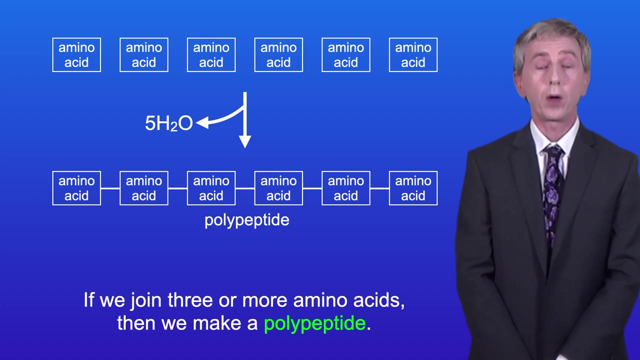 it contains two amino acids bonded together. This reaction takes place in ribosomes, which is where amino acids are synthesized in cells. The reaction is catalyzed by a specific enzyme, and we look at that in a later video. Now, if we join three or more amino acids, then we make a polypeptide and 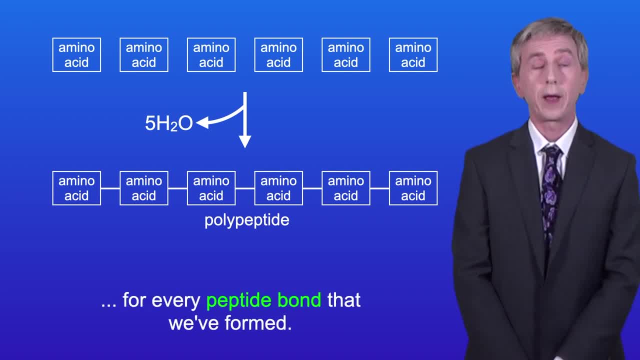 I'm showing you that here. As you can see, we've made one molecule of water for every peptide bond that we formed. Now I should point out that polypeptides often consist of hundreds of amino acids joined together. Okay, so, as we've seen, a peptide bond is formed in a condensation reaction. 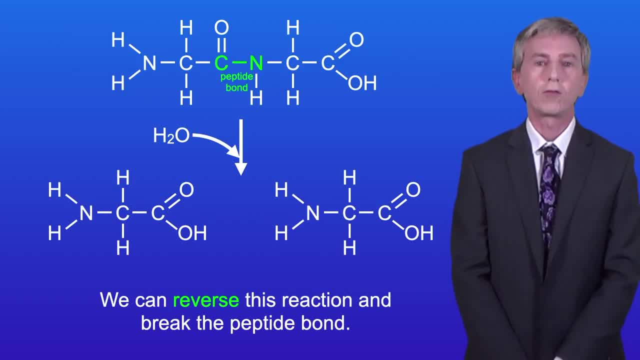 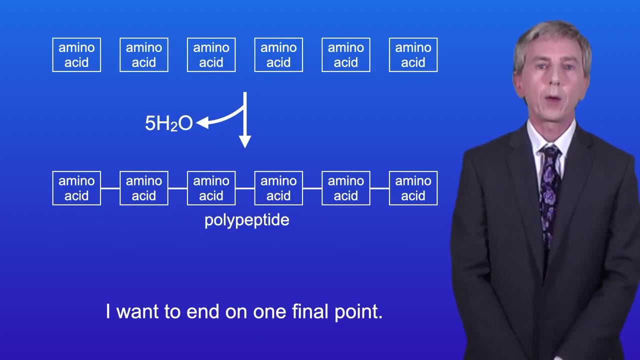 A molecule of water is produced. Now we can reverse this reaction and break the peptide bond, and to do that we need to add back a molecule of water. This is called a hydrolysis reaction, and this reaction is carried out by protease enzymes in the digestive system. Okay, I want to end on one.